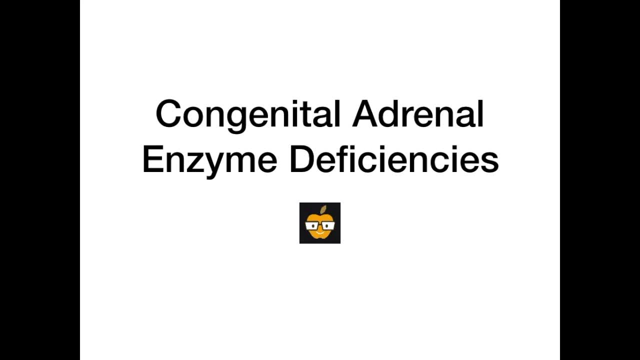 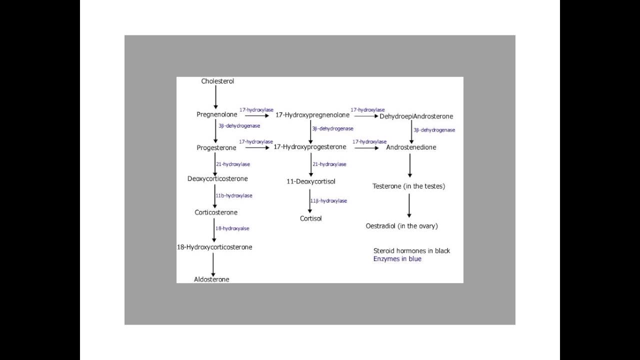 In this video I'm going to be talking about the congenital adrenal enzyme deficiencies. This is brought to you by Dirty Medicine. Now I know what you're thinking: Oh, Dirty, no, not the adrenal enzymes. Relax, we are not going to need to refer to this diagram. 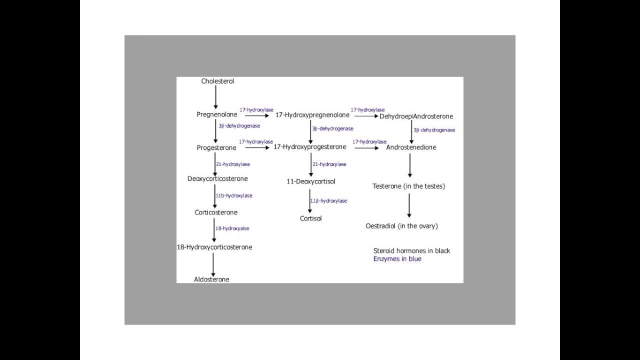 I'm putting this here because this is probably what jumped into your brain right As soon as I said adrenal enzymes. you probably thought, oh my god, I need to finally memorize that stupid enzyme flowchart that you see on this slide, that I always skip through in all of. 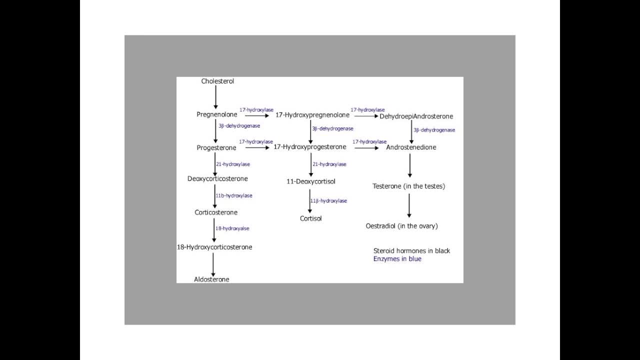 my review textbooks and in all of my question banks. Well, that's the truth, guys. You absolutely don't need to know this And unless you're going to be an endocrinologist or a very, very, very nerdy, maybe even PhD level internal medicine doctor, there's really no point in. 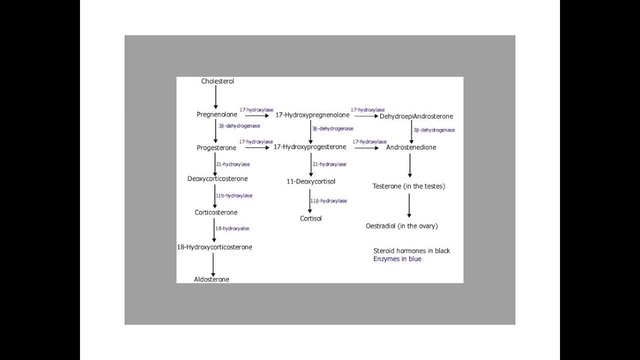 memorizing this, So throw it out of your brain. take that piece of paper that has this on it, crumble it up, throw it in the toilet and flush that puppy, because you don't need to know this. Instead, what I'm going to focus on is what you do need to know and what you need to know specifically for your congenital adrenal enzyme deficiencies. Now you probably want to know what the key to your brain is and what's the main cause of this deficiency. Well, there's a lot to know about this. So, first of all, if you remember. you probably know the basics of what it is, So it's called the first aid or whatever you're using, And it's called the first aid or what's the main cause of this deficiency? And you might have noticed that it's called the first aid, but it's 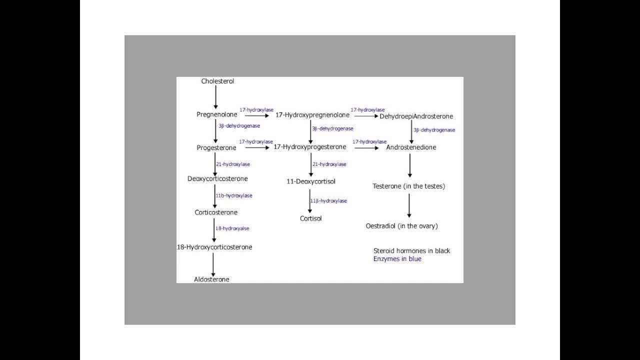 actually called the first aid. So first aid is the first aid for all the steps and levels of USMLE and COMLEX. Now if you flip through first aid or whatever review textbook you're using, you'll probably notice that there are normally three major adrenal enzyme deficiencies. 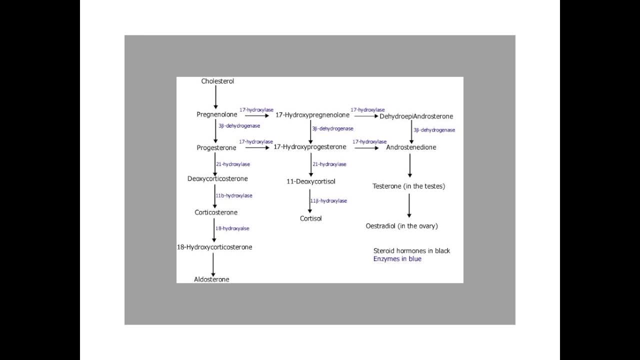 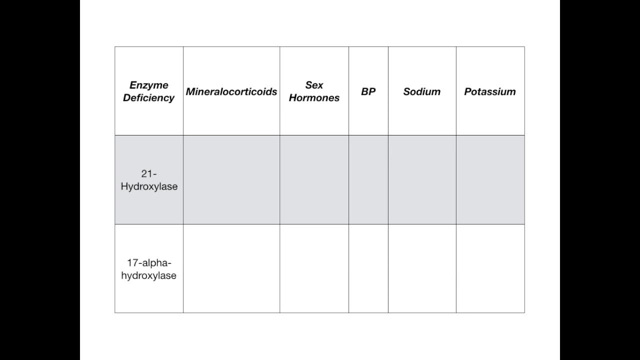 that get mentioned And only two of those are really particularly high yield And those are shown on this slide: the 21 hydroxylase deficiency and the 17 alpha hydroxylase deficiency. The other one is very low yield and I don't recommend that you commit it to memory unless 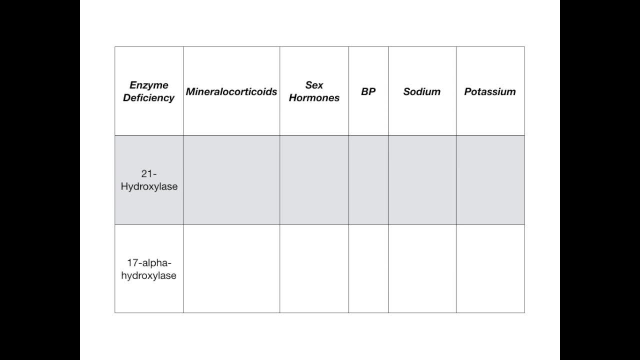 you have some extra brain space lying over at the end of this lecture, But, for all intents and purposes, what I think you should take away from this video is how to differentiate 21-hydroxylase deficiency from 17-alpha-hydroxylase deficiency. 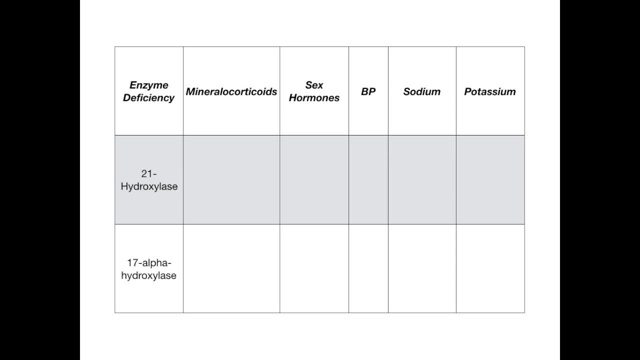 And specifically what the test writers are going to expect you to know, and what's actually pretty high yield- is being able to discern what happens to the mineralocorticoids, what happens to the sex hormones, what happens to the blood pressure, the sodium and the. 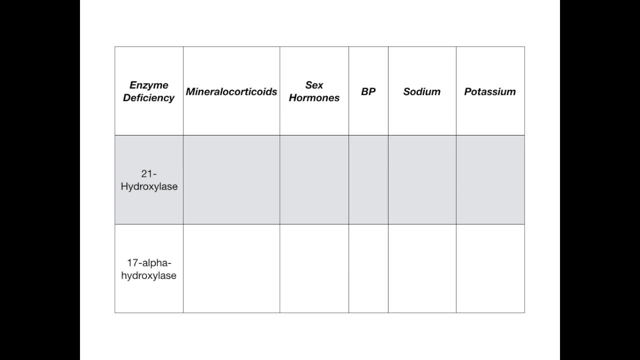 potassium in each of these two disease states. Now, if you feel slightly overwhelmed right now because you're looking at this chart and you already don't quite understand the adrenal enzyme deficiencies and now you're seeing all these things that you need to know, that I'm telling you are high yield, I want you. 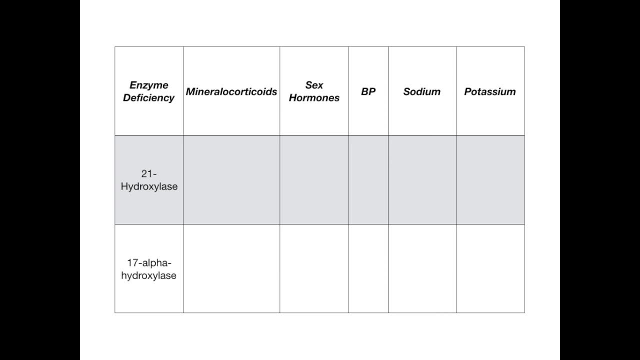 to relax, because the way that you're going to learn this, if you watch my video today, is with a pretty awesome mnemonic. It is so simple: You just tell yourself a little story And you'll learn it. You'll learn all of this information in no time. 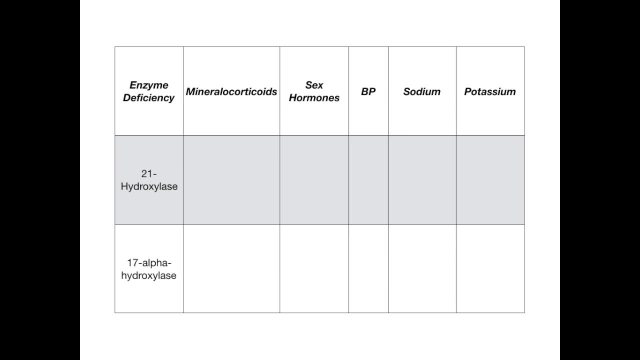 So the way that my mnemonic works is that I need you to imagine somebody who just wants to go to college. All they want to do is go to college. And the way that we're going to use this mnemonic is that we're going to look at the 21-hydroxylase. 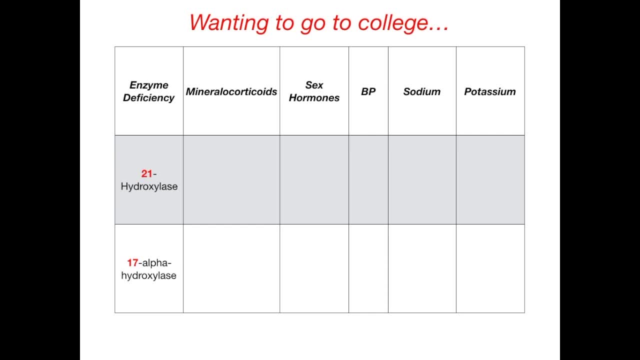 deficiency and take the number 21 out, And that'll be our 21-year-old. And then we'll look at the 17-alpha-hydroxylase deficiency and take the number 17 out and have a 17-year-old. So in this story, 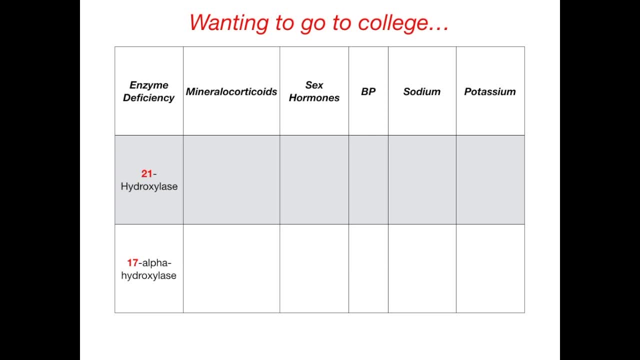 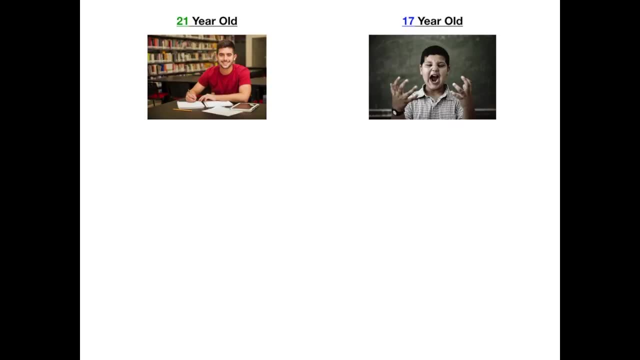 You've got a 21-year-old college student and a 17-year-old high school student, And remember: the goal is to go to college. Everybody wants to go to college, So here's how I'm going to set up this mnemonic for you. 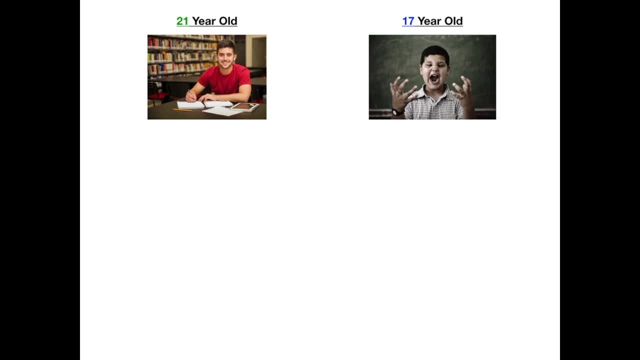 So we've got our 21-year-old and he's happy as a clam, right, Because he's in college. He made it. He gets to study, learn what he wants to learn, go out and party with his friends. He's living it up. 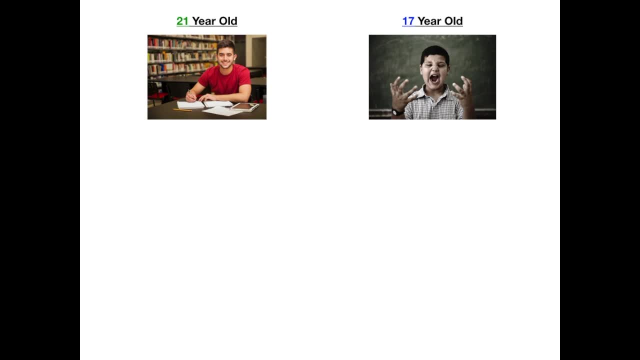 He's happy. But our 17-year-old high school student: he is miserable because he's still stuck in high school. All he wants to do is go to college. So here we go: We've got our 21-year-old, who's in college, and very happy, and our 17-year-old, who's not. 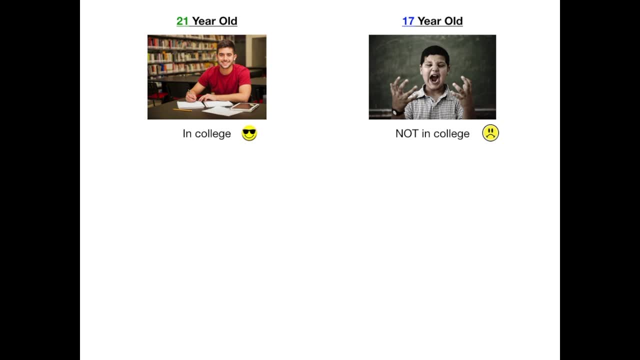 in college yet. So he's pretty upset. Now, what does this mean? Well, when you're 21,. you're in college, you're manly. right, You've made it. You're a senior in college, you're manly. 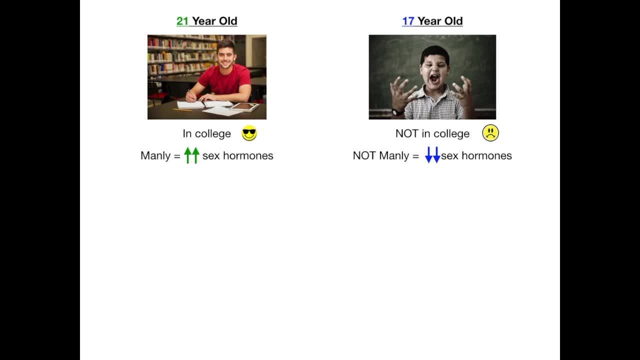 So that stands for increased sex hormones for the 21-year-old. But the 17-year-old he's not manly yet because he's still a little baby. He's in high school. His voice probably still cracks, to be honest with you. 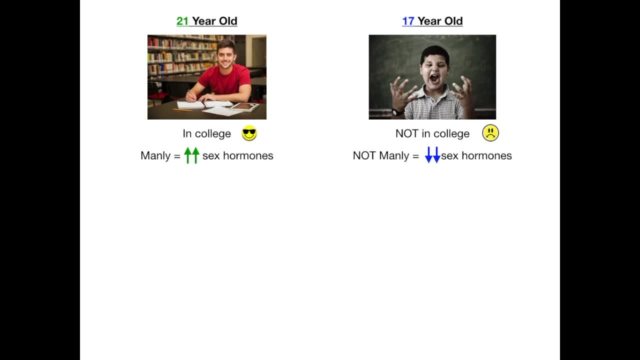 So in the 21-hydroxylase deficiency There's increased sex hormones, because when you're 21 and in college you're manly. But in the 17-hydroxylase deficiency, that's the 17-alpha-hydroxylase deficiency, there's 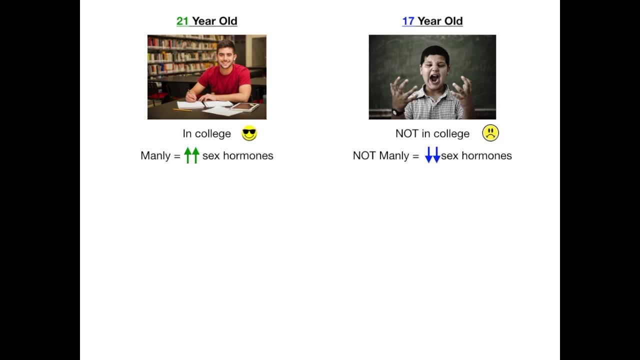 decreased sex hormones. because you're still in high school, You're not manly yet. So, 21 in college: manly: increased sex hormones. 17 still in high school, not manly yet- decreased sex hormones. Now let's move on. 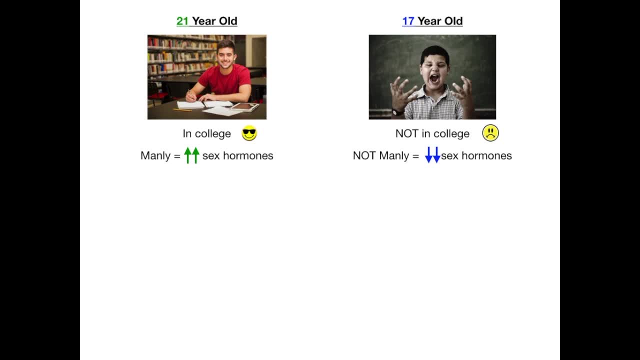 So we've talked about sex hormones and now let's talk about mineralocorticoids. So because the 21-year-old Is really happy, he's not salty, And because the 17-year-old is really upset, he is salty. So we say that you're really salty if you're really angry and upset and pissy. 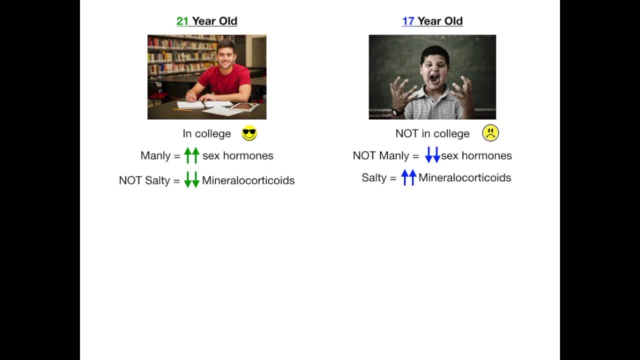 So the 21-hydroxylase deficiency is not salty, which is to say that there's decreased mineralocorticoids because the mineralocorticoid is aldosterone and that is responsible for salt. So in the 21-hydroxylase deficiency we've got a 21-year-old student really happy and 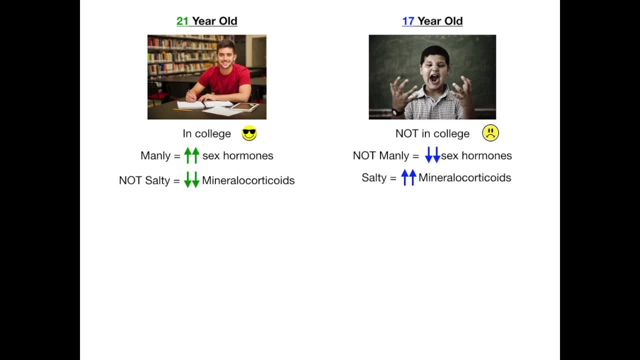 therefore not salty. So there's decreased mineralocorticoids. But in the 17-alpha-hydroxylase deficiency, the student who's still in high school and so upset that he's not in college yet, he's really salty. So there's increased levels of mineralocorticoids. 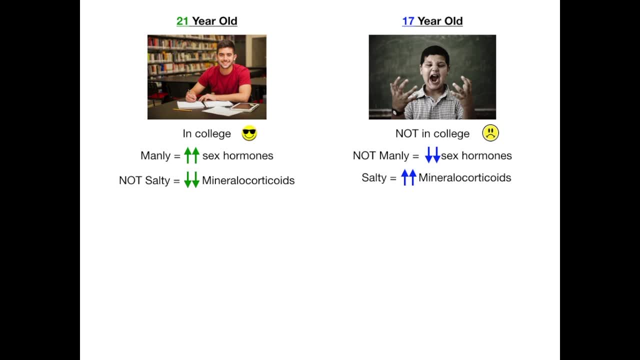 Now, if you have a little bit of background knowledge about what a mineralocorticoid is right, We're talking about aldosterone. You should know what aldosterone does in the body. Aldosterone increases sodium, increases blood pressure and decreases potassium. 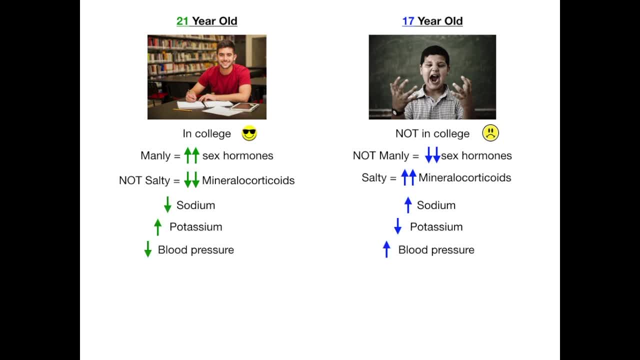 So in our 21-hydroxylase deficiency, where there's decreased mineralocorticoids, also known as decreased aldosterone. that means that there's decreased sodium and therefore decreased blood pressure and increased potassium. So in our 21-year-old college student who's not salty and therefore does not have aldosterone. 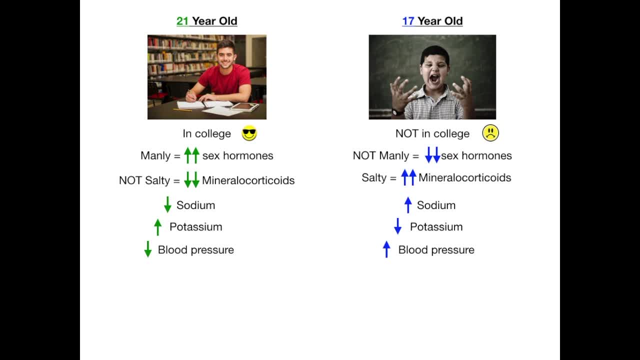 or has decreased aldosterone. there's decreased sodium, increased potassium and decreased blood pressure. But in the 17-alpha-hydroxylase deficiency It's the 17-year-old, very salty high school student- right, He's salty. 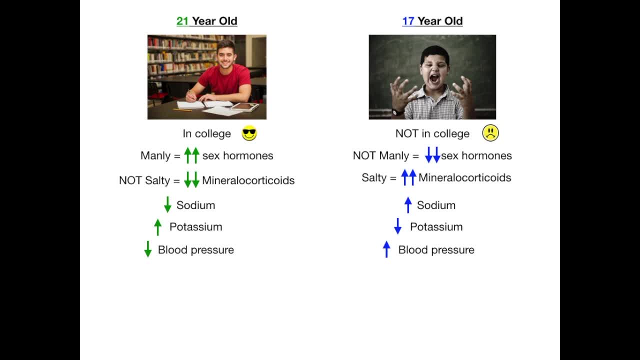 He just wants to go to college. So that means there's increased levels of mineralocorticoids, which is increased aldosterone. And what happens when aldosterone is up? Well, sodium is up and therefore blood pressure is up and potassium is down. 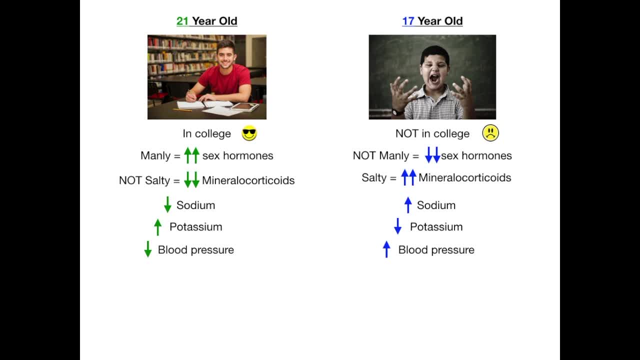 So just by taking the numbers out of the two deficiencies right- 21 out of 21 hydroxylase and 17 out of 17 alpha hydroxylase- and creating this stupid mnemonic, this stupid story that I made up years ago. the 21-year-old is happy because he's in college, but the 17-year-old 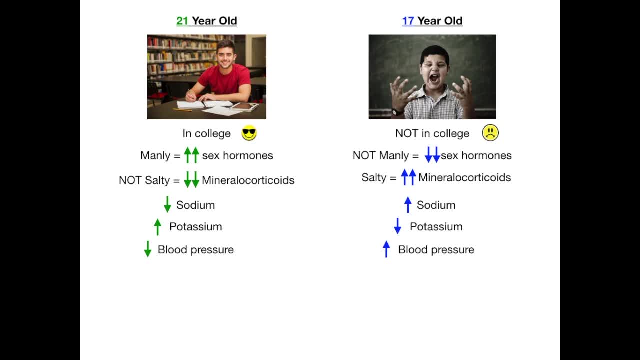 is pissed off because he's still in high school and just wants to go to college. By doing that, by extracting those numbers, you can learn everything you need to know to differentiate the two adrenal enzyme deficiencies. So go through this story one more time and make sure that it really hits home in your 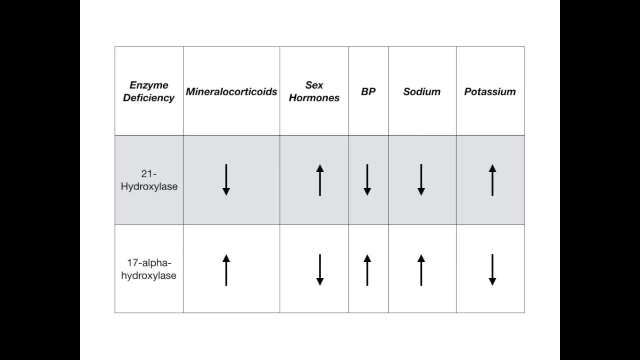 brain and that you can understand, Because once you do, it's really easy to fill in this chart. And let's just prove it to you by running through the story one more time. So we've got two main adrenal enzyme deficiencies: the 21 hydroxylase deficiency, which will 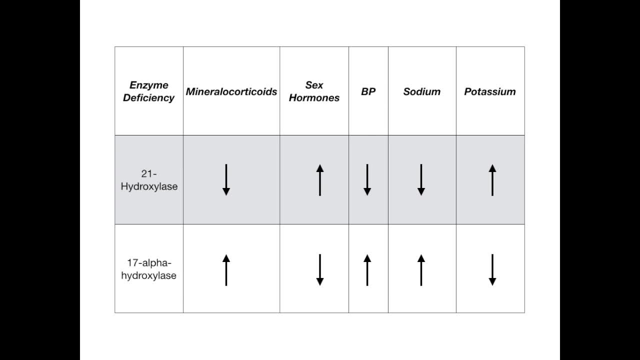 in our story, be the happy 21-year-old who's already in college, because he's 21,, and the 17 alpha hydroxylase deficiency, which is our 17-year-old, And when you're 17,, you're usually not yet at college. 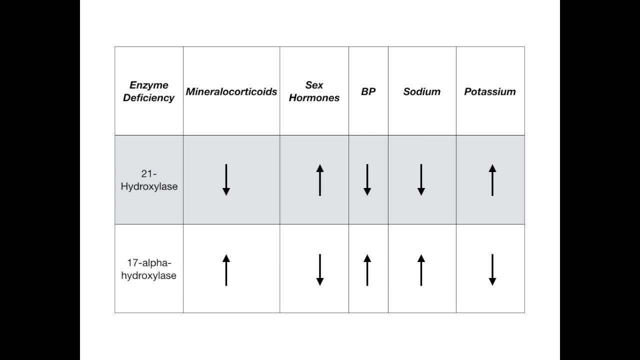 So you're still stuck in high school and you're pretty upset because you're still in high school and you just want to go to college. So the 21-year-old, He's in college, He's manly And therefore his sex hormones are up. 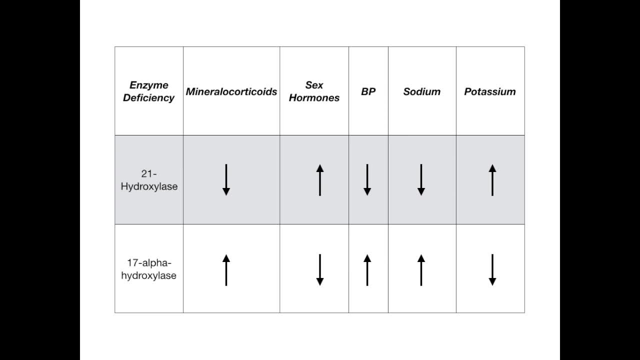 But the 17-year-old, you know, he's still a little babe. He's in high school, His voice might still be cracking, He's learning how to talk to women, He's still discovering himself. So the sex hormones are going to be down in the 17 alpha hydroxylase deficiency. 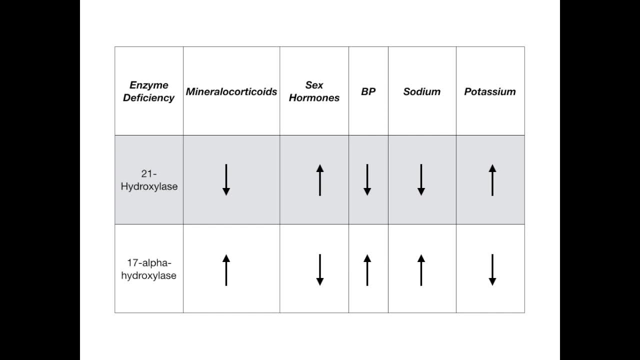 Now, because our 21-year-old is really happy: he's not salty, So he has decreased levels of salt. So mineralocorticoids are down, which means aldosterone is down. And if aldosterone is down, that means that sodium and therefore blood pressure are. 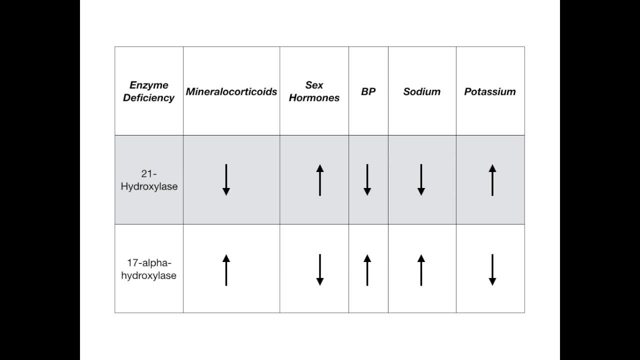 both down but potassium is up. But in the 17-year-old he's so salty because he just wants to go to college He's like: why the hell am I still in high school? And because he's salty, his salt or his mineralocorticoids or his aldosterone are up.